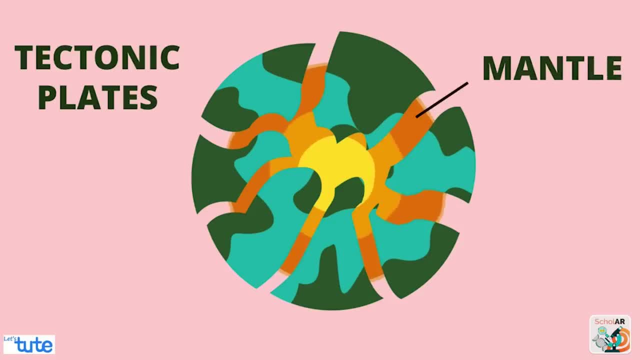 are placed on a plate called a tectonic plate. These plates are placed on a plate called a tectonic plate. These plates are placed on a hot, partially molten layer of earth's mantle. This is the reason why these pieces are continuously moving. They are moving as you are watching this video. These 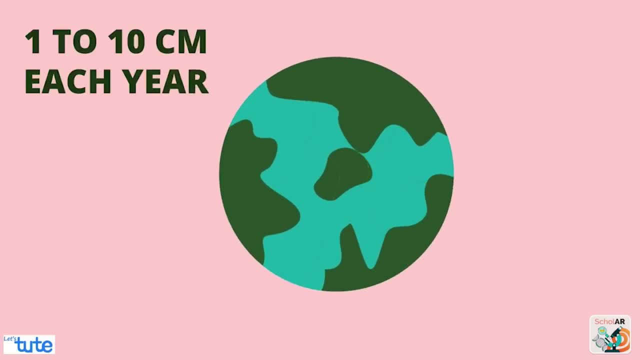 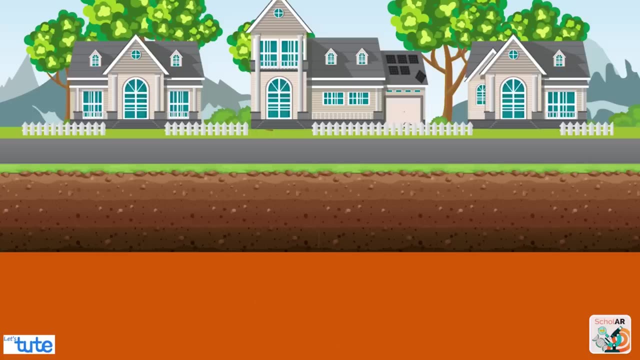 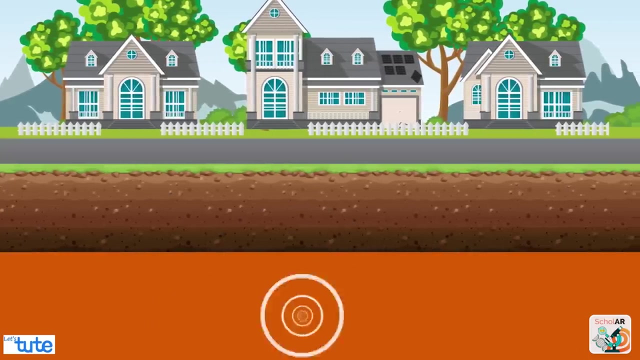 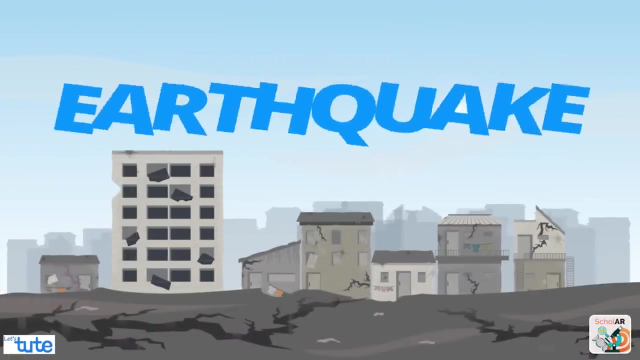 plates move around 1 to 10 cm each year. But don't worry, not all these movements can be felt by us. Sometimes these movements are extremely strong and can be felt like a lot of vibrations under your feet, Or it can also destroy an entire city. That's called an earthquake. 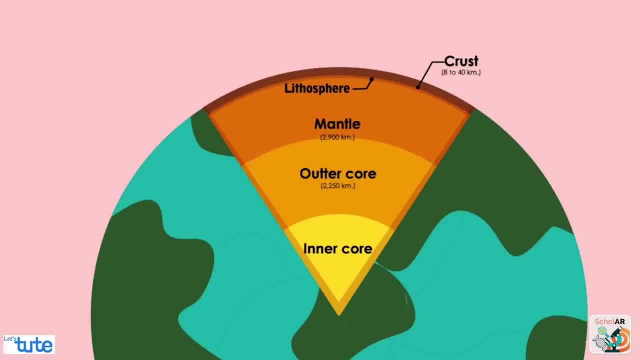 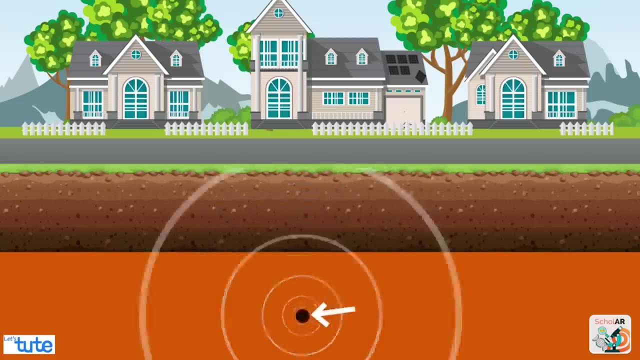 The earthquakes occur in the lithosphere region of the earth. An earthquake generates underneath the earth and this releases the energy across. The point at which the earthquake occurs under the earth is called hypocenter, and the exact place above it, at the surface of the earth, is called 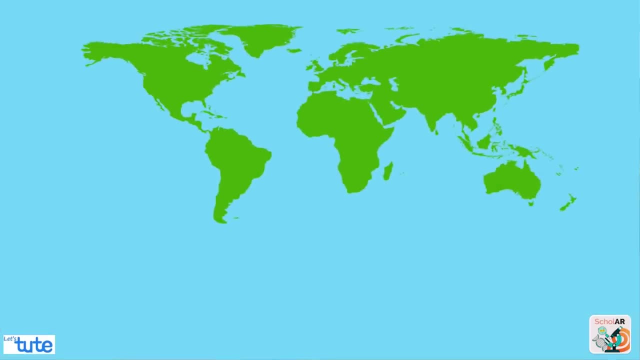 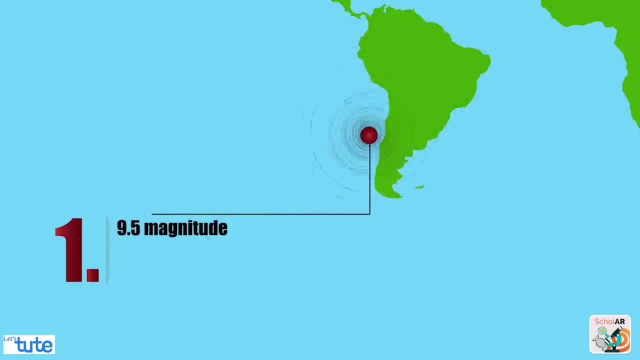 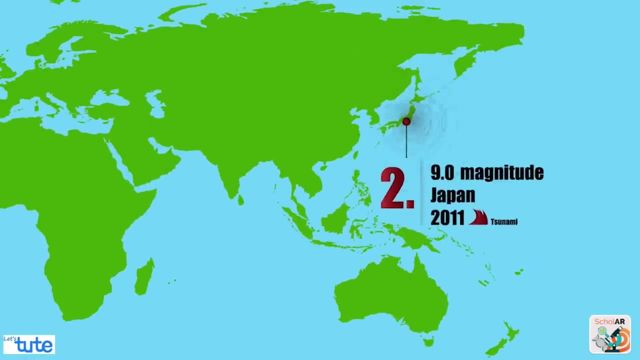 epicenter. The most horrifying earthquake recorded till date was of magnitude 9.5 out of 10.. This happened in Valdivia in southern Chile in 1960.. Another one that happened in Japan, in Tohoku region, was of magnitude of 9.0, which happened on March 11, 2011.. This earthquake caused a massive 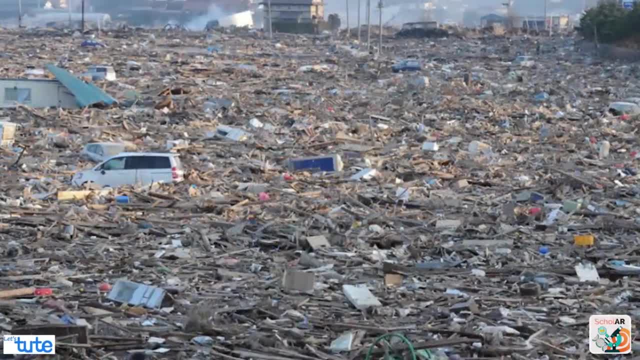 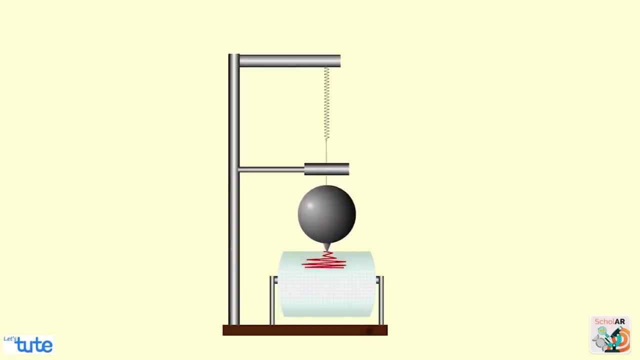 and enormous damage to the earth. The earthquake caused a massive and enormous damage to the earth. It caused damage and destruction and took nearly 16,000 people's lives with him. Geologists use a device that can sense the waves created by the movement of the tectonic plates. 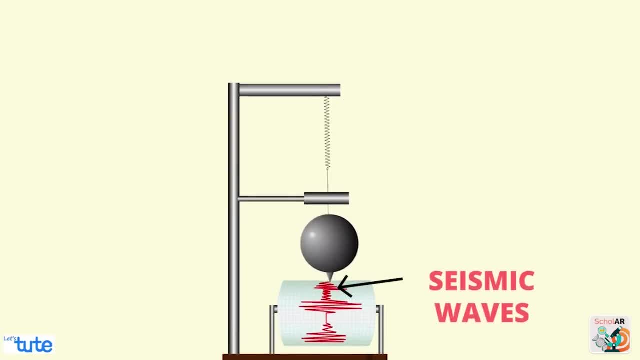 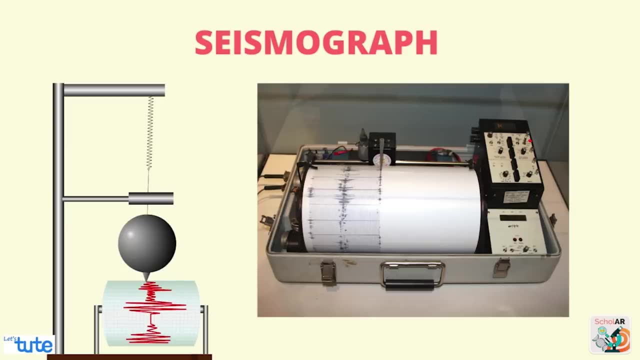 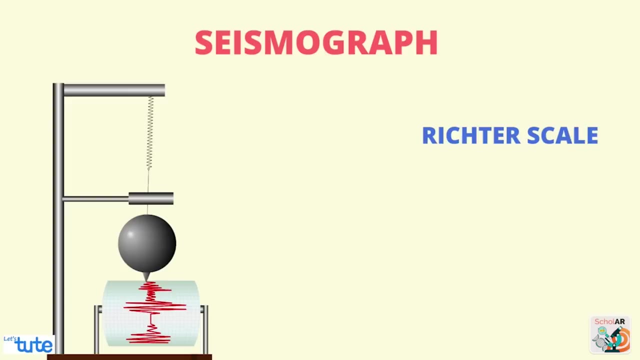 These waves are known as seismic waves and the device is called a seismograph. The earthquake events are scaled according to the magnitude of the shock and are known as Richter scale. This magnitude relates to energy released during the earthquake. Magnitude is expressed in absolute. 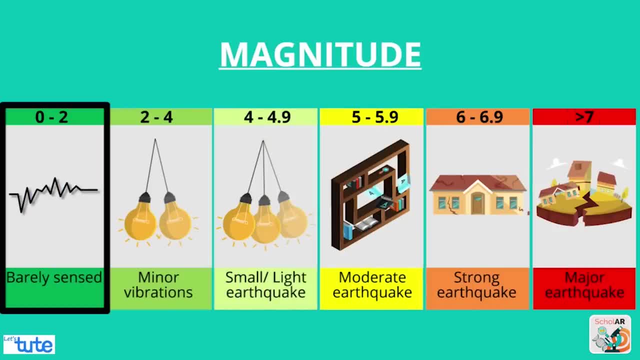 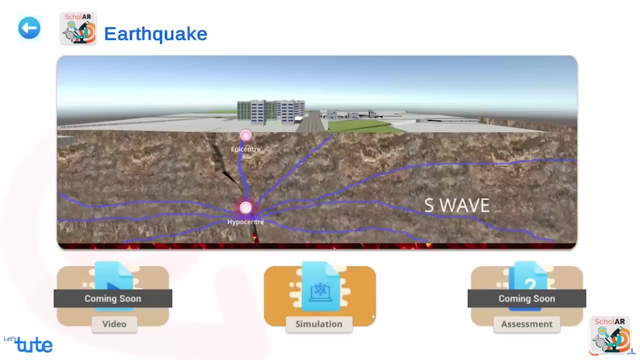 number 0 to 10, where zero is lowest, where people feel nothing, and 10 being the highest, that can create severe destruction and loss of life over a large. In order to know more about earthquake, let's jump to the simulator. We can see on the screen is the inner core of the earth. 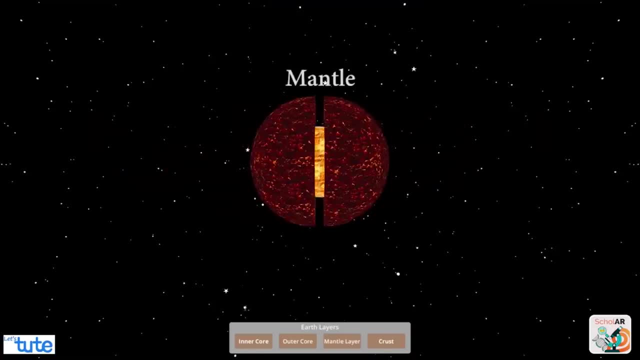 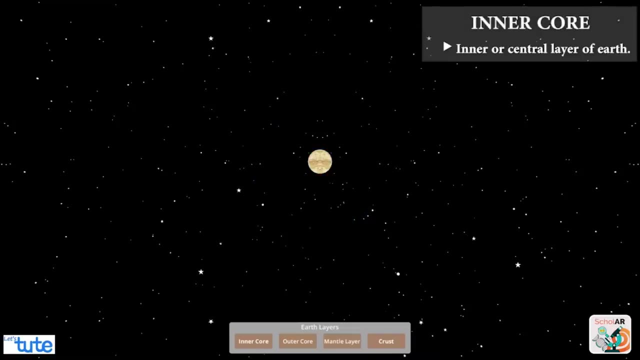 And then we have outer core, mantle and crust. The inner core, as the name suggests, is the innermost layer or the central layer of earth. It is like a solid spherical ball in nature, with a radius of 1250 kilometers. The temperature of earth's core ranges between 4500 to 5500 degrees. 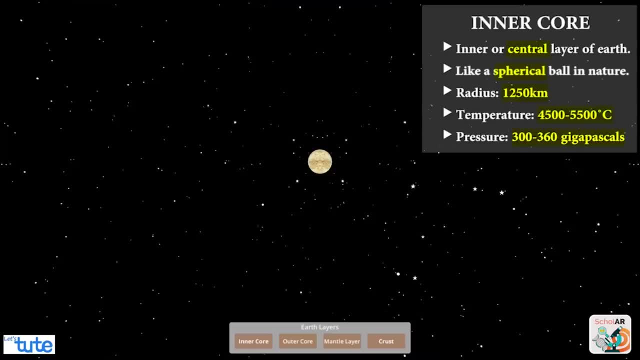 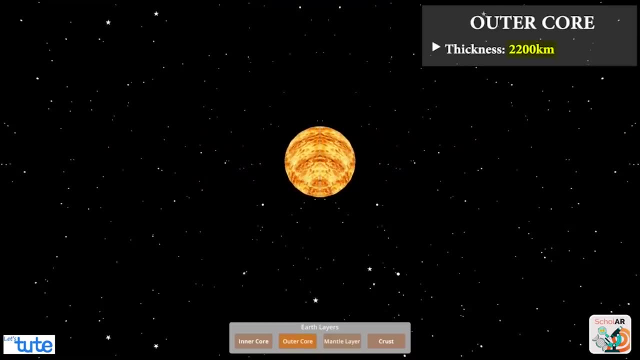 celsius. The temperature of earth's core ranges between 4500 to 5500 degrees celsius, facing a pressure of 300 to 360 gigapascals. Next is outer core. It is of about 2200 kilometer thickness and has a temperature similar to inner core, that is, of 4500 to 5500. 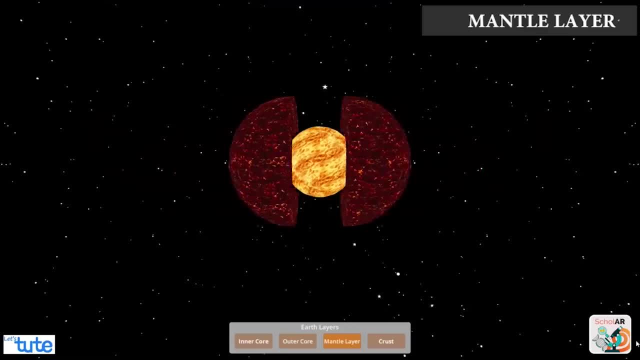 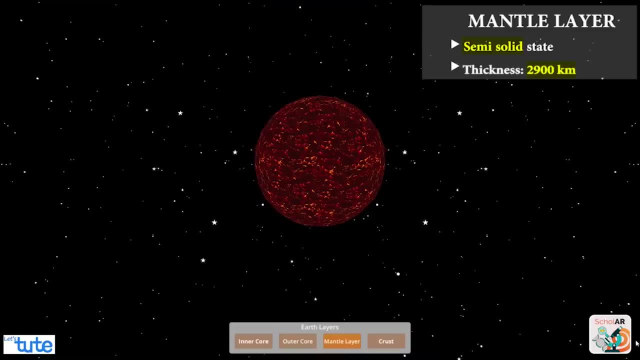 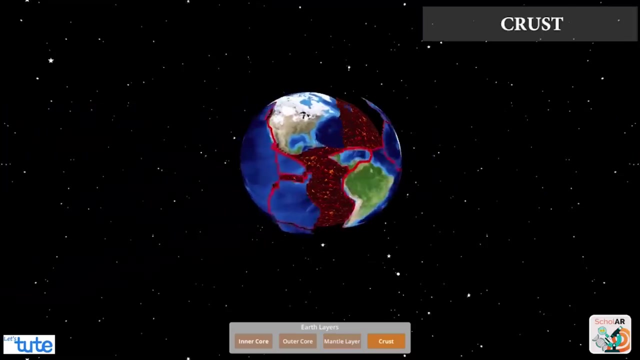 degrees celsius. Then we have the mantle layer, which is the semi-solid state of about 2900 kilometer thickness. This layer makes around 84 percent of earth's total volume, And the last layer is the crust, which is like an apple skin when compared to other layers. 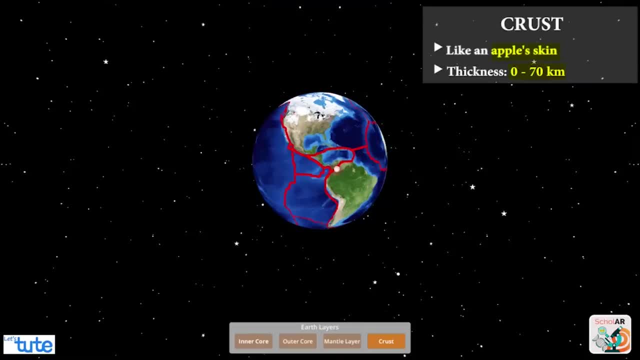 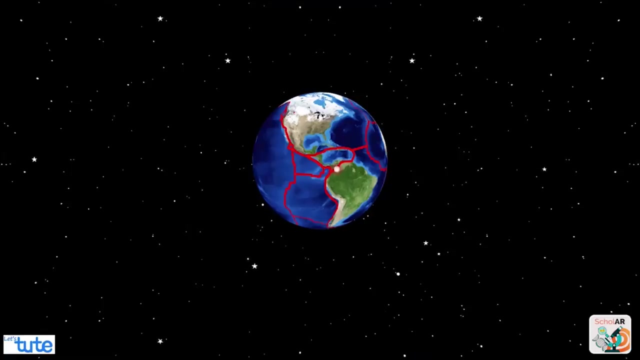 Runs from 0 to 70 kilometers in thickness, which is specifically 8 kilometers under sea to 32 kilometers under continents, and this is only 1 percent of the earth's total mass. Now we can see that there's a grayish white dot. Let's click on that. 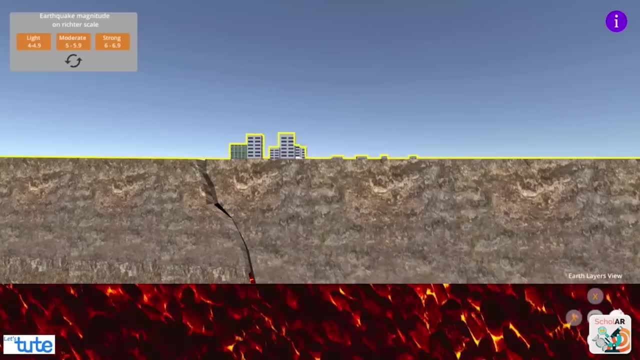 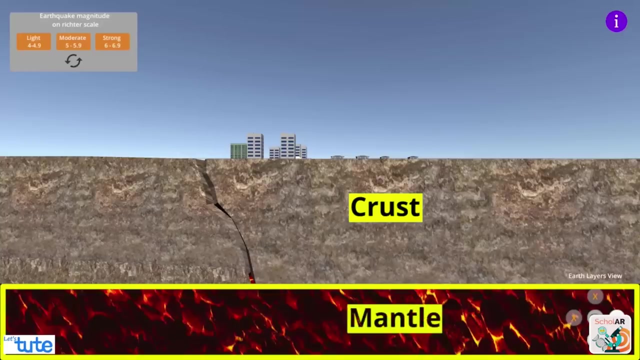 We can see a small town when we see this in the street view and then when we click on layer's view, we can see earth's layer. the grayish in color is called as crust and the one in reddish color is called as mantle. On the left hand corner side we can see we have a small box that says: 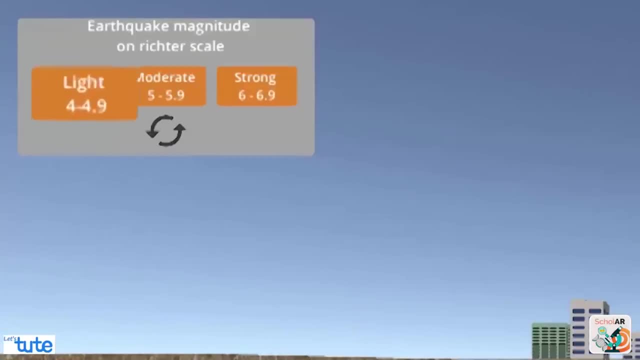 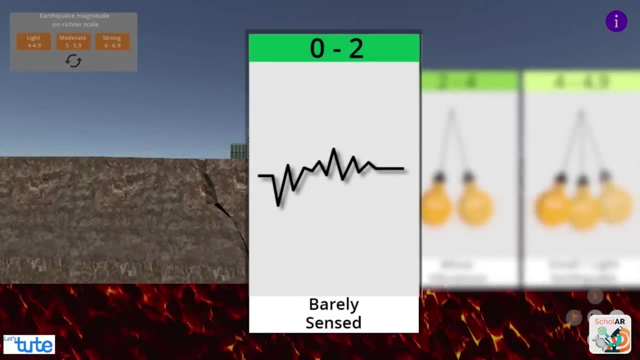 earthquake magnitude on richter scale with three buttons, that shows the magnitude of the earth's magnitude, which is equal to 32 millimeters per second in color, And then we have an earth's of the earthquake. if the intensity is between 0 to 2, it can be barely sensed. 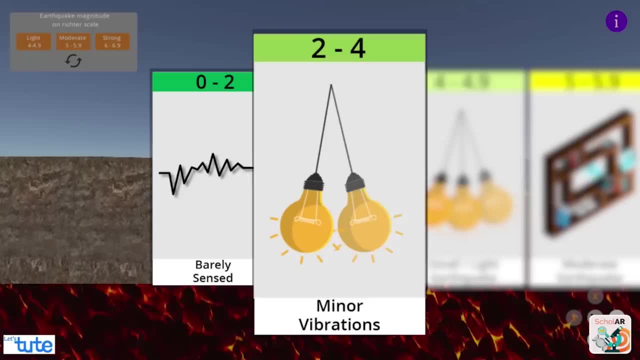 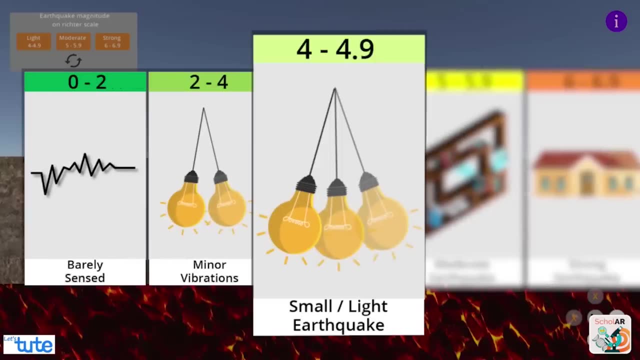 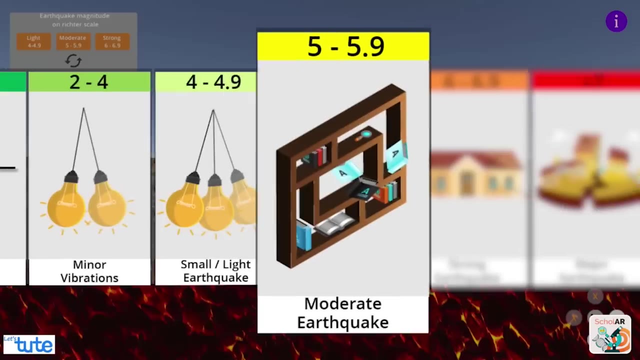 when the intensity is more than 2 and less than 4 we can feel minor vibrations and sense it a little. from 4 to 4.9 it is considered as small or a light earthquake. range from 5 to 5.9 are considered moderate earthquakes and from. 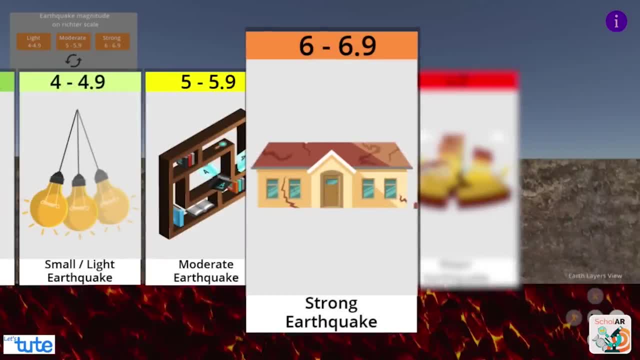 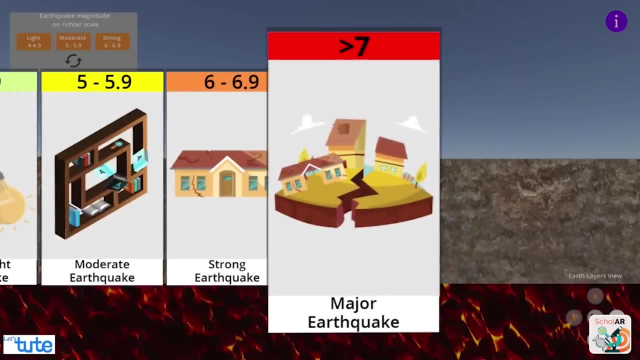 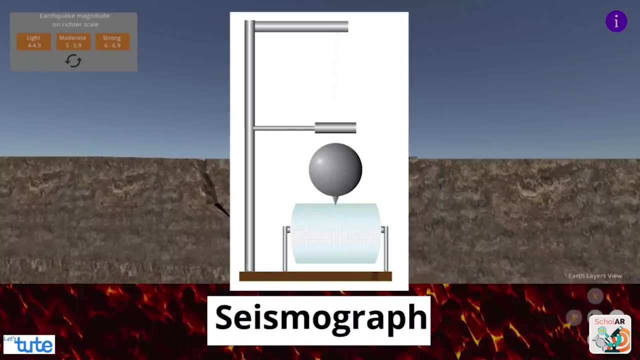 the range 6 to 6.9 are considered as strong earthquakes. in some time we will see how much damage these magnitudes can do, and anything about 7 is considered as major earthquakes which can destroy cities and continents. these readings are recorded on a seismograph. now let's hit the 4 to 4.9 magnitude to see how this. 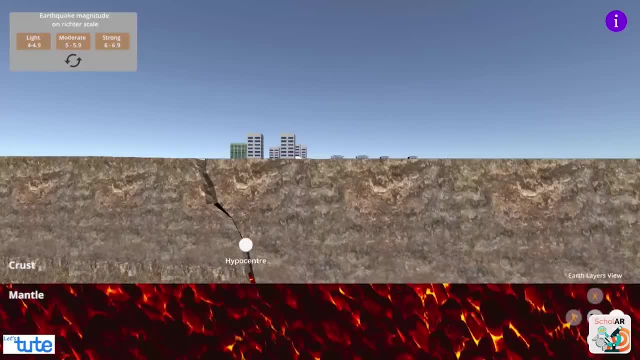 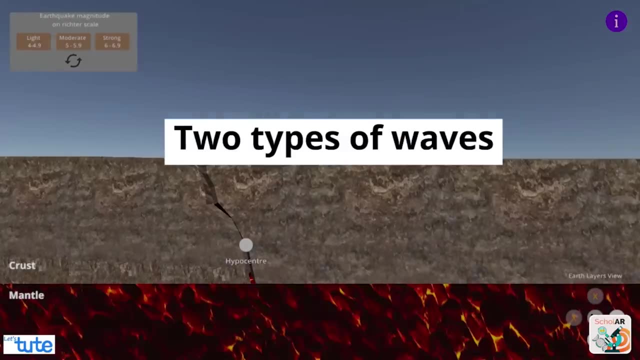 earthquake will react. earthquake happens. we can see the earthquake starts from a point called a hypocenter inside the earth. during an earthquake, two types of waves are formed. one is called body waves and the other are called as surface waves. let's see what are called as body waves. body waves are the waves that moves through the 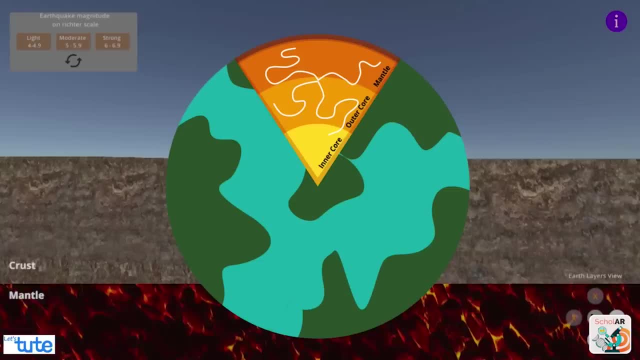 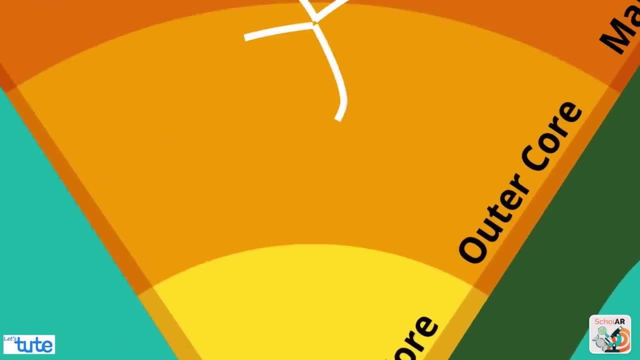 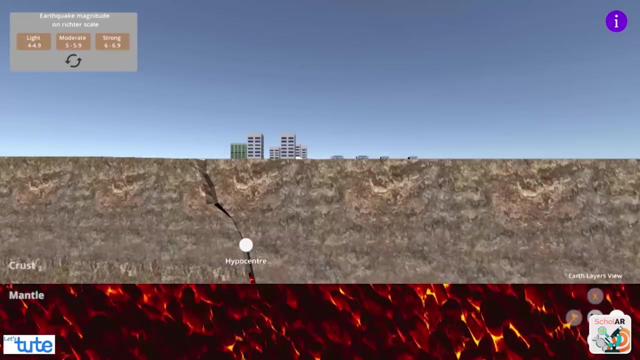 interior of the earth and through the body of the earth, and hence the name waves. when these body waves move, these waves come across the surface rocks and generate the surface waves. let's see in detail about these body waves and surface waves. from this point, that is, hypocenter, waves are released. these waves are called primary waves or p waves. 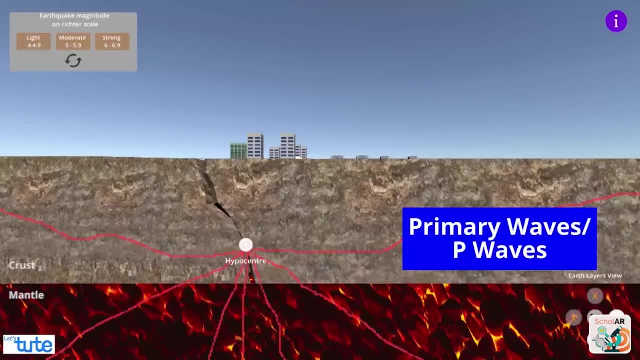 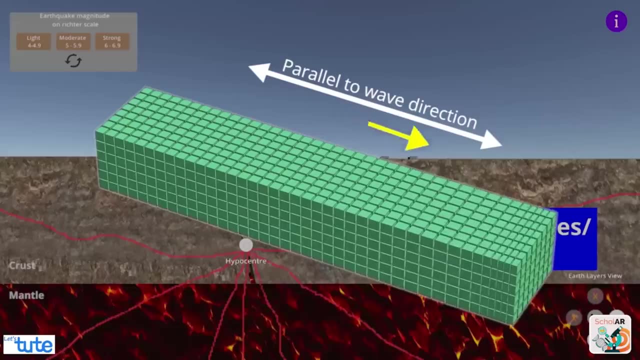 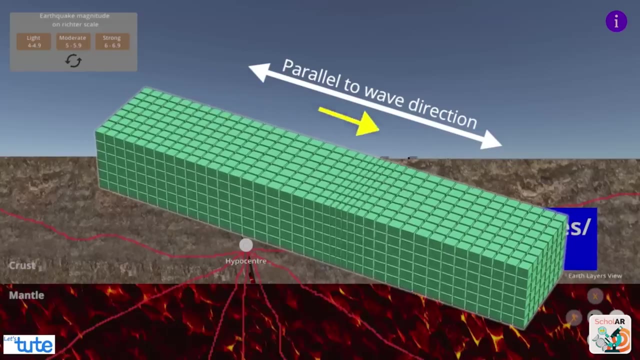 now, what are these p waves? p waves are seismic waves. these are the waves that shake the ground back and forth in the same direction and the opposite direction, as the direction of the wave is moving, which is similar to the movement of these sound waves. this is how a p wave looks like. these p waves. 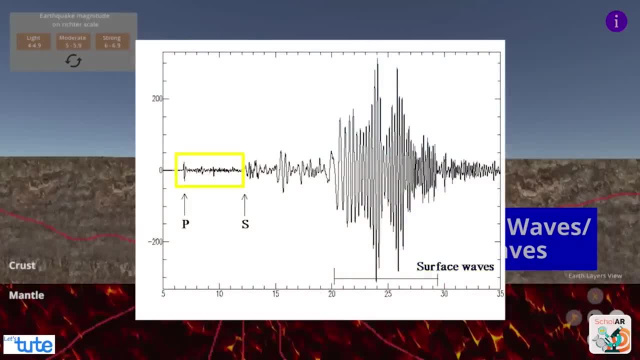 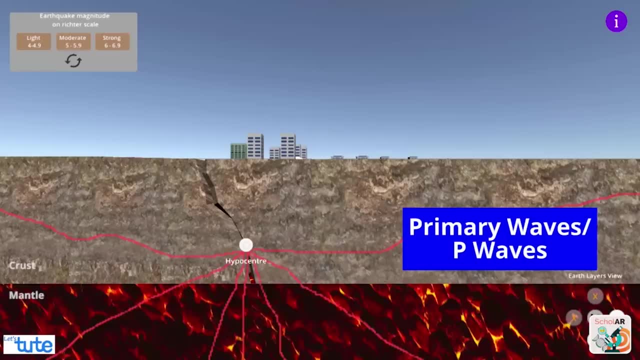 are the first to be recorded on a seismograph. now, after a fraction of second, when these p waves hit, the rocks closer to the surface gives rise to new seismic waves after the p wave. the second type of waves we saw are called as secondary waves or dermatoc комментарia. 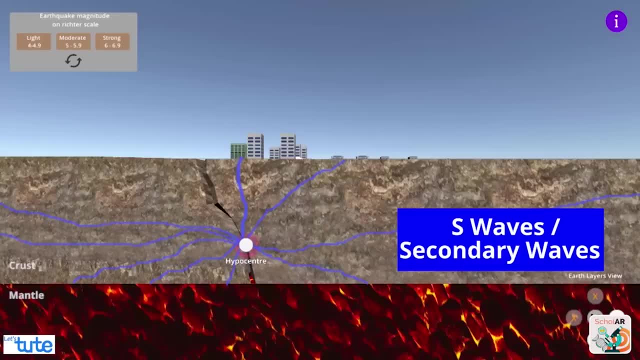 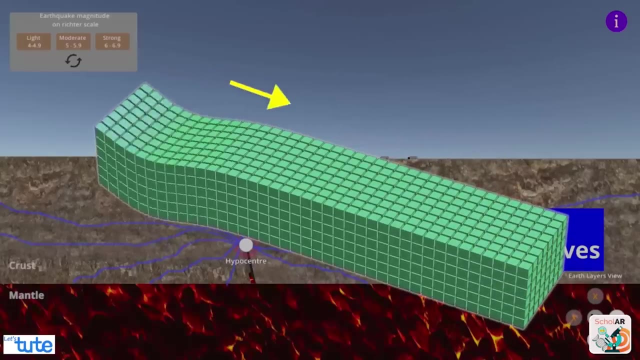 waves S waves that were recorded on a seismograph were called secondary waves. These waves are towards the earth's crust and these are tremors and vibrations that we feel. These waves are the wave motion in a solid medium, where the medium move perpendicular to the direction of the wave. 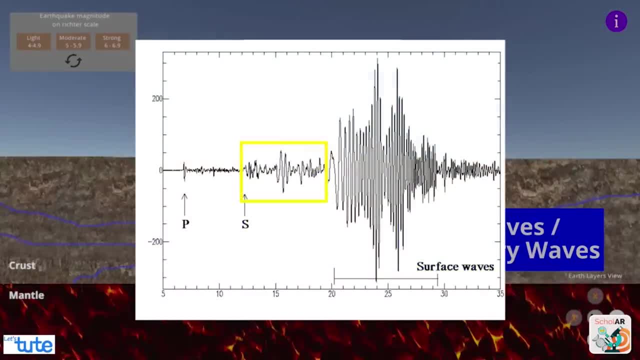 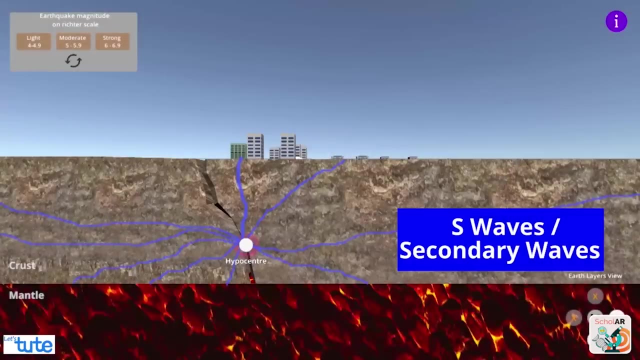 After the p wave, these s waves are recorded on a seismograph. Now these S waves hits the surface and starts the earthquake. The point at which the earthquake originates on the surface is called an epicentre. After the P and S waves comes the surface waves, which are the most destructive waves. 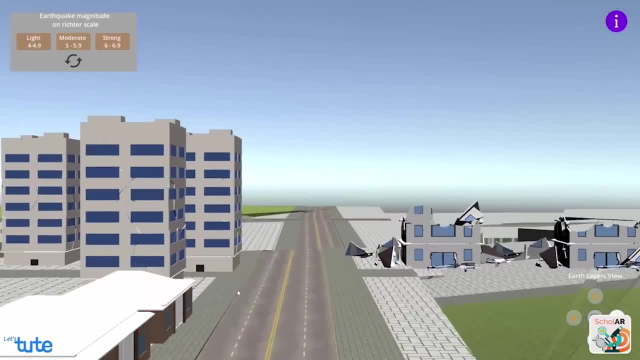 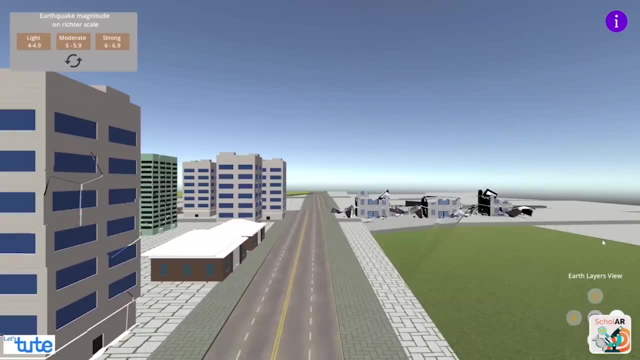 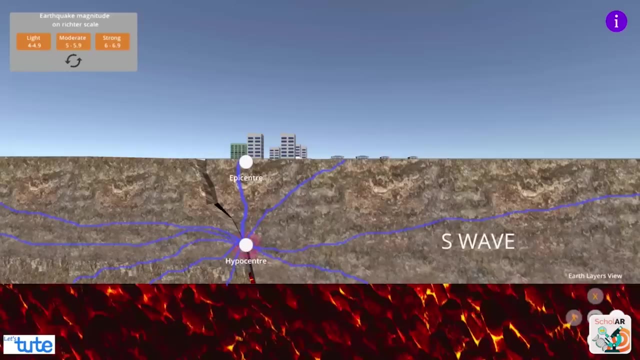 as they cause the movement or the displacement of the rocks, which leads to falling of structures and causing harm to life. Let's once again see the formation of P and S waves. We can see that an earthquake of this magnitude- that is, between 4 to 4.9, causes the damage. 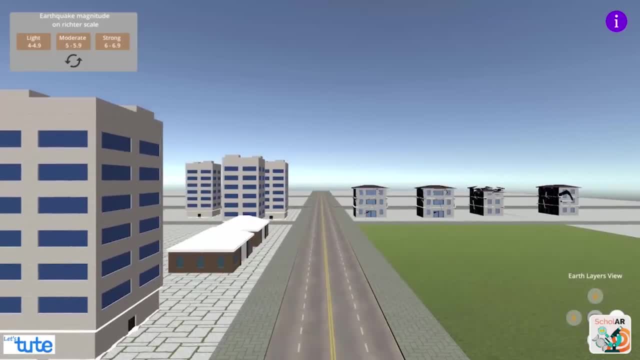 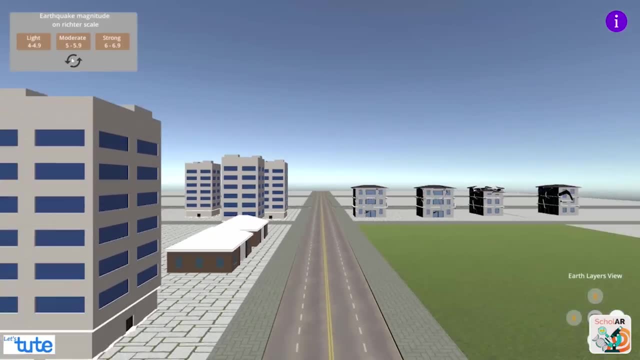 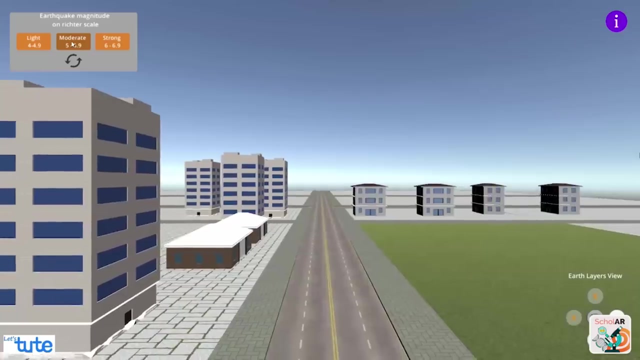 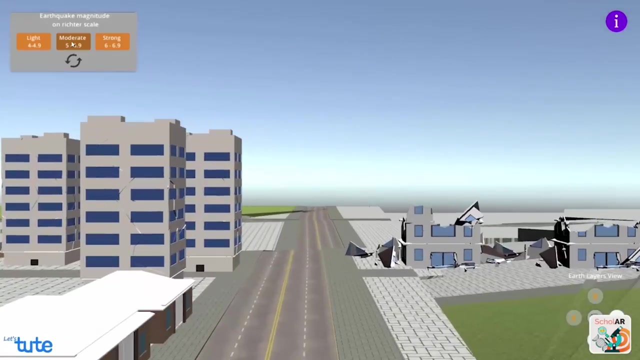 to nearby small houses, but the buildings are okay. Let's see what happens when the magnitude is between 5 to 5.9.. Let's reset and then hit the button Okay. Whoa, that's quite some damage. The small houses are shattered and the buildings also have cracks. 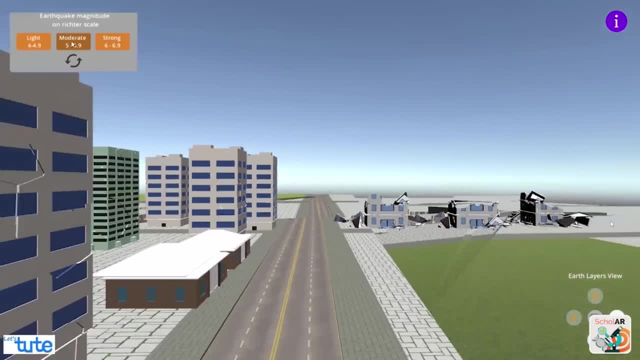 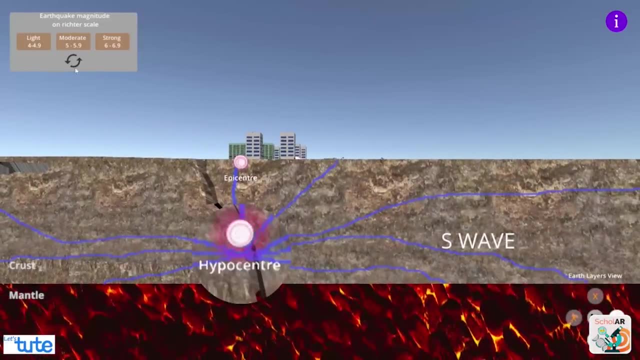 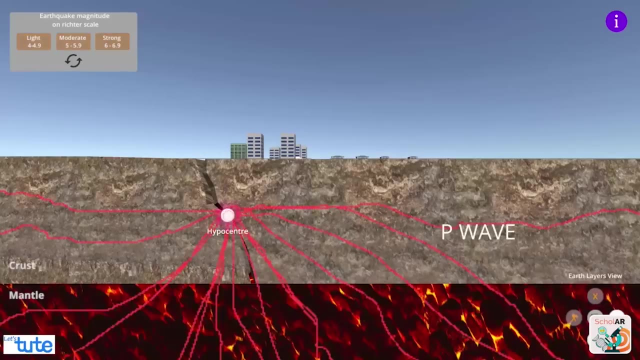 We can also see that the road is also cracked now. One more thing to notice is that the higher the magnitude, the closer the hypocentre is to the epicentre. Notice this: when we move to 6 to 6.9 magnitude, The damage is enormous. 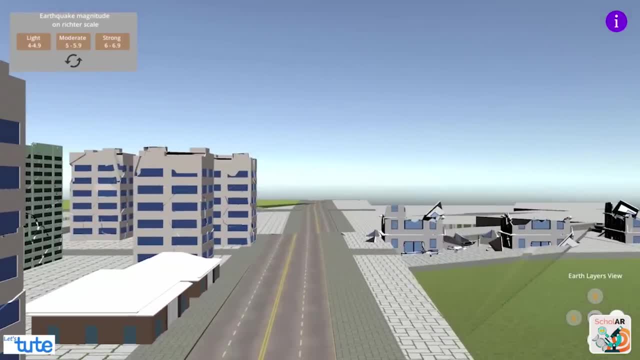 Buildings are almost broken, roads are cracked and small houses are collapsed. Earthquakes can really be extremely damaging natural calamity. If this is the case when magnitude is limited to 7, imagine how 9 and 9.5 might even look. 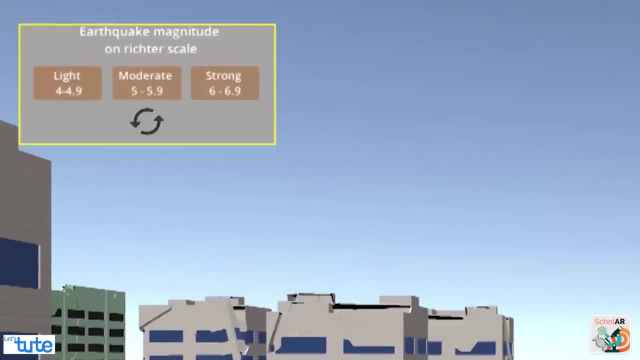 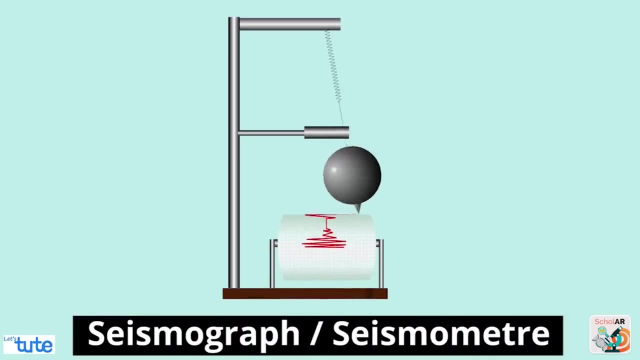 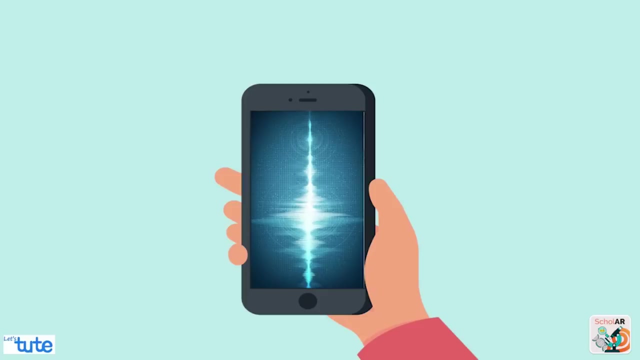 Since these are quite commonly occurring magnitudes, we have studied them in this simulation. It is exciting to see. It is extremely difficult to predict an earthquake based on a seismograph, which is also known as a seismometer, But even our smartphones can now detect these seismic waves and scientists can use this data to predict earthquakes and warn people. 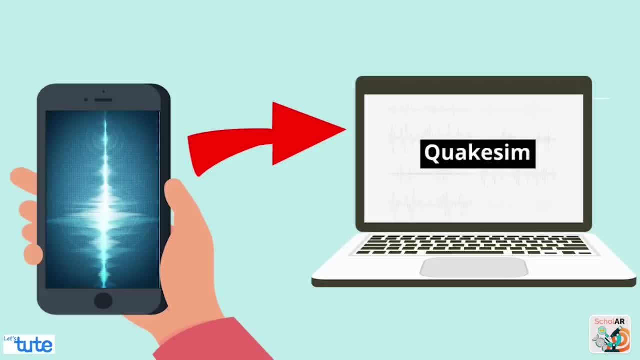 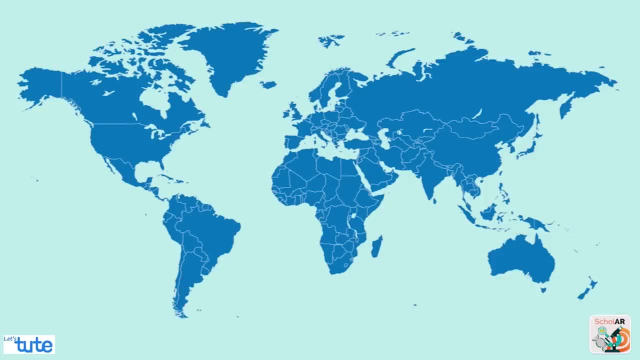 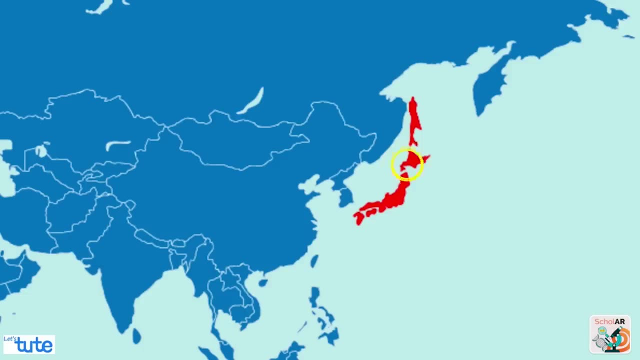 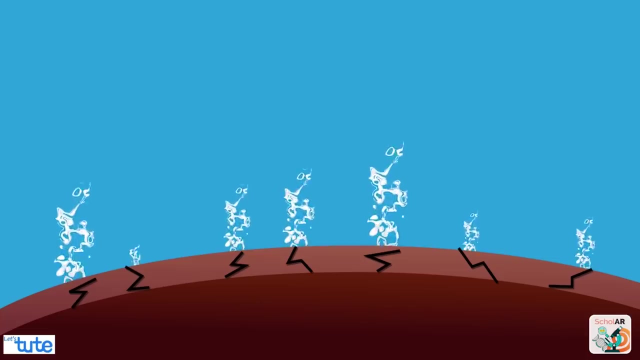 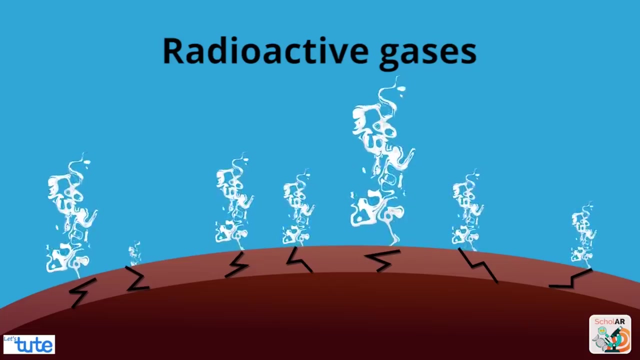 NASA can use this information in the Quakesim software, which can use this data to generate more efficient information. Recent studies showed that, before an earthquake, nearby regions record very high concentrations of radioactive pair, radon and thoron. This happens because, right before the earthquake, these gases are released on the surface from small cracks and if we can detect these gases, we can predict a quake at least 7 days in advance. 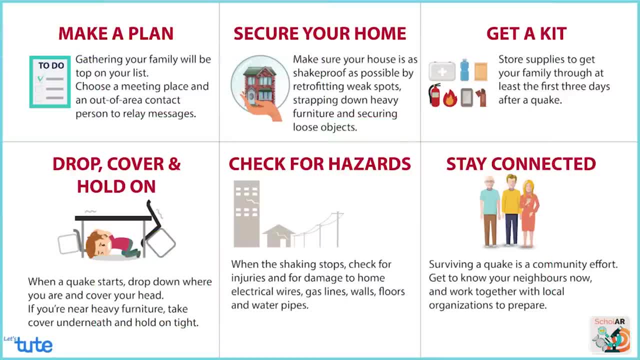 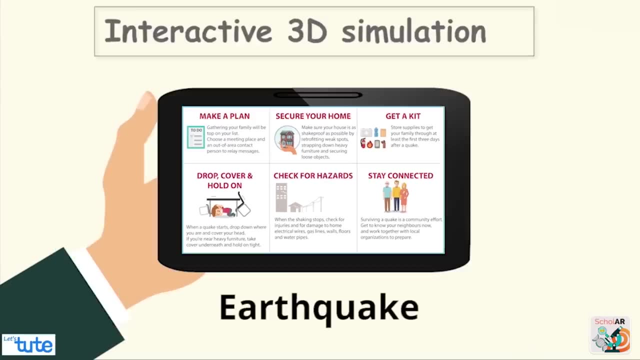 Well, here are some tips that can save you time In case of an earthquake. Till then, keep yourself safe and see you in the next session. Well, I hope you have enjoyed this session. This session is based on an interactive 3D simulation called Scholar, developed by Esquivel. 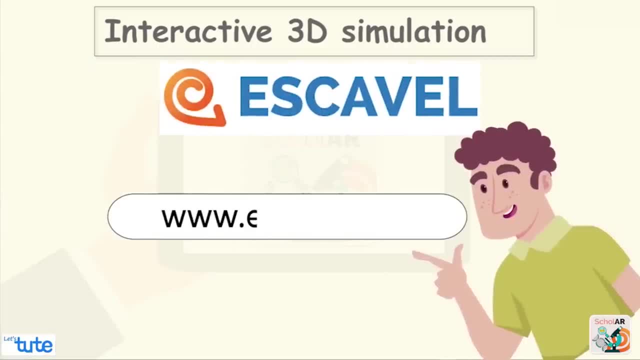 Visit wwwesquivelin to request the download of the software application to try this out yourselves. If you have enjoyed this video, please like, share and subscribe to our channel. Thank you. If you liked this video, hit the like button. 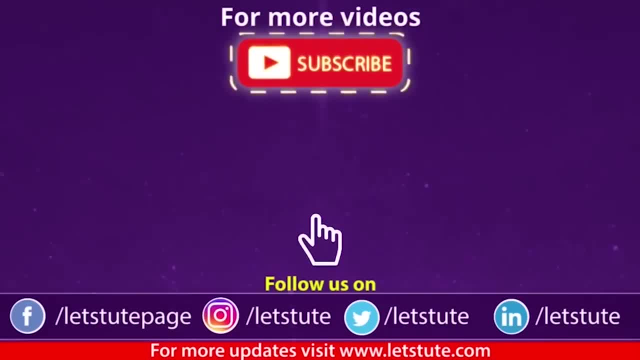 If you have any queries, comment down. and yes, don't forget to hit the bell icon and never miss another update from Let's Tut. Keep watching, keep learning and follow your curiosity, Thank you.